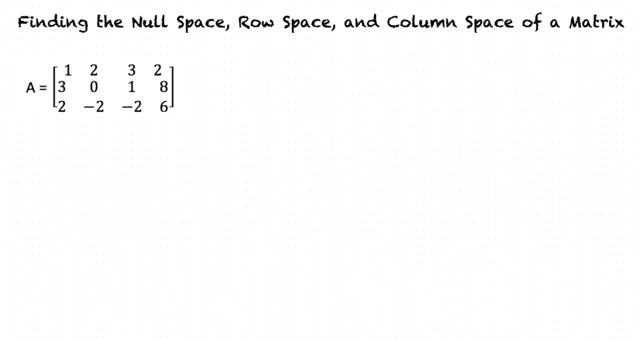 2, 6.. For this matrix, we must find the null space, the row space and the column space. Okay, what is our first step in finding these? To begin, we must put our matrix into the matrix equation. The matrix equation is written as: matrix A times X is equal to 0.. Now we 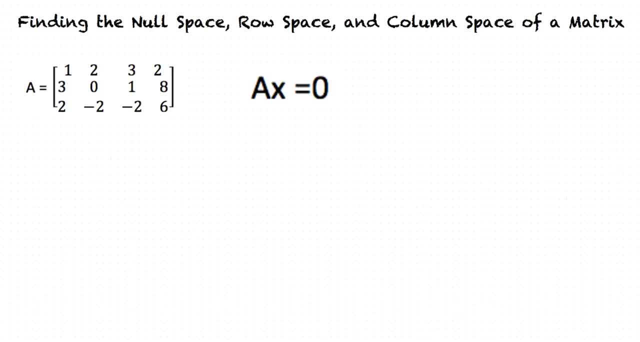 can insert our matrix into the matrix equation. This will look like: row 1, 1, 2, 3, 2, row 2, 3, 0, 1, 8, row 3, 2, negative 2, negative 2, 6, times row 1, X of 1, row. 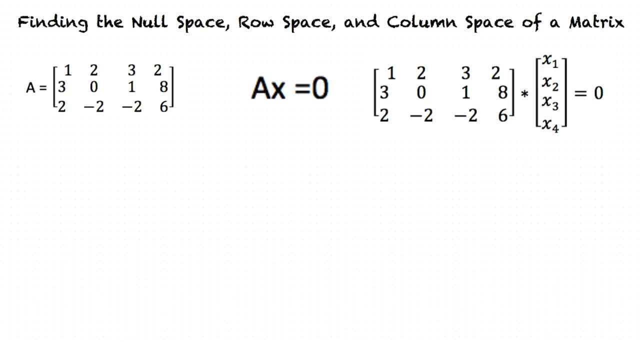 2, X of 2, row 3, X of 3, and row 4, X of 4 is equal to 0.. From here we must put our matrix A into reduced row echelon form. We do this using the RREF function on our calculator. Once we take the RREF of A in 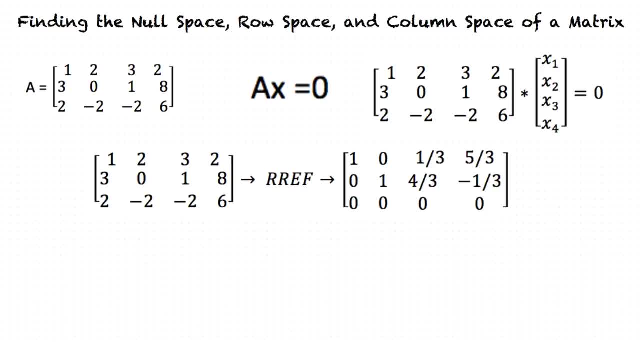 our calculator we will get row 1, 1, 0, 1. third, 5 thirds. row 2, 0, 1, 4 thirds negative: 1 third. row 3, 0, 0, 0, 0.. We will first find the column space of the matrix. We will 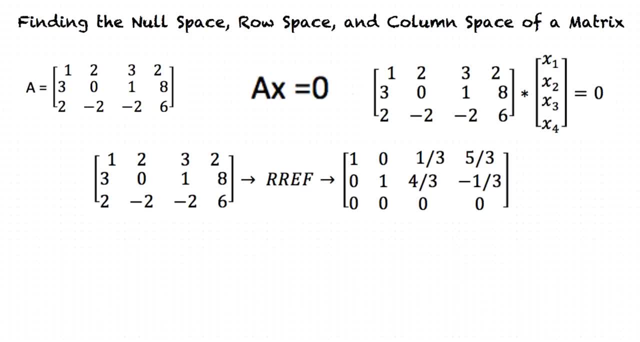 do this by finding the columns with the 1's as pivot points. With this one, the column 1 and 2 have pivot points. From here we take columns 1 and 2 of matrix A as our column spaces. This gives us: column 1 is equal to 1, 3, 2, column 2 is equal to 2, 0, negative 2.. Now 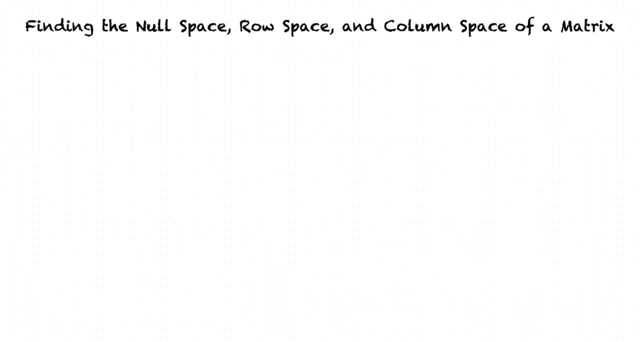 that we have found the column space, we need to find the row space next. We will first look at the matrix A. To do this, we must once again look at the matrix in reduced row echelon form. The reduced row echelon form of matrix A is row 1, 1, 0, 1 third, 5 thirds. 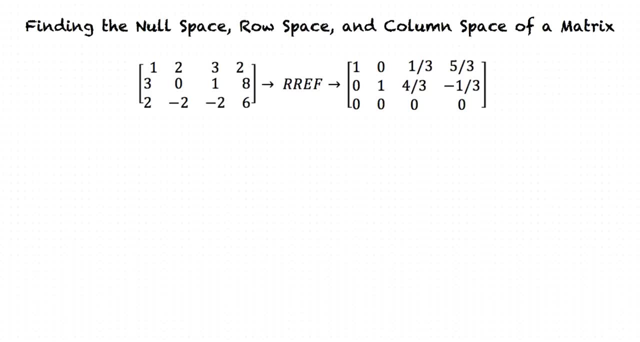 row 2, 0, 1,, 4 thirds negative 1 third, and row 3, 0, 0, 0, 0.. Now, what do we do, though? Once we have a matrix in reduced row echelon form, we must take the 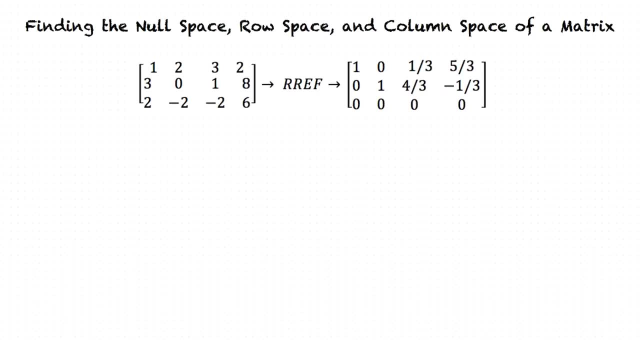 that have 1 as a pivot point. Our row spaces will be derived from the reduced row echelon form of the matrix. For this one, rows 1 and 2 contain our pivot points. This means our row space will be row 1, 1, 0, 1, third, 5. 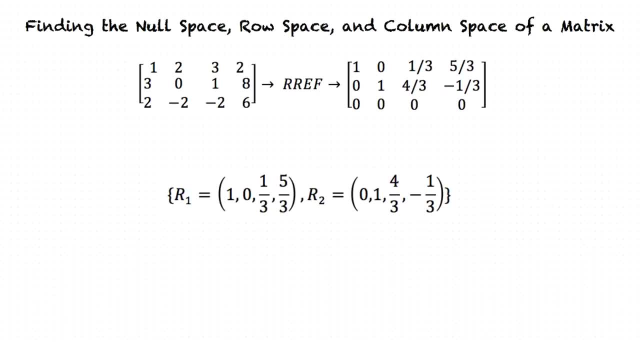 thirds: row 2, 0, 1,. 4 thirds. negative: 1 third. Now we have to find the null space of the matrix. We will once again use the reduced row echelon form. This will look like: row 1, 1, 0, 1 third. 5 thirds. row 2, 0,. 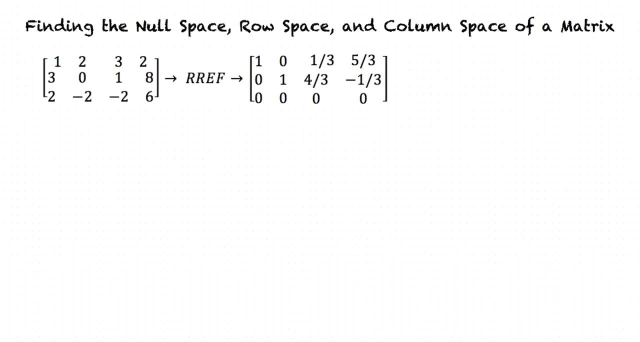 1, 4 thirds, negative 1 third and row 3, 0, 0, 0, 0.. We have reduced row echelon form, So now what do we do To begin finding the null space? we? 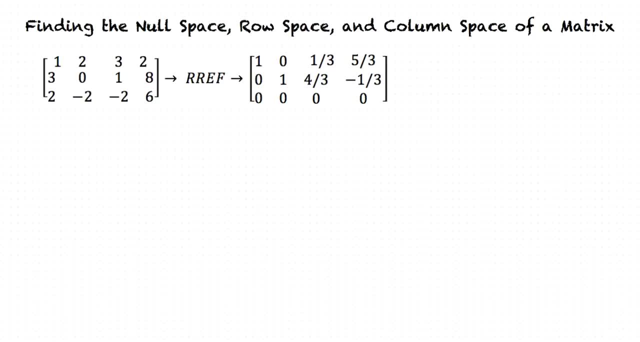 must parameterize the solution. We will start by solving for x3 and x4.. Since these are free variables, we can insert any arbitrary number. This means that we must select a variable that could be anything. This gives us: x3 is equal to t and x4 is equal to s. 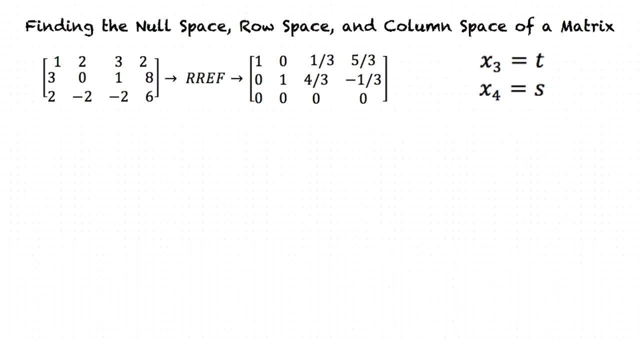 Now we need to solve for x1 and x2.. We do this the same way that we would solve an equation For x1,. we would need to solve the equation x1 plus 1 third, x3 plus 5 thirds: x4 is equal. 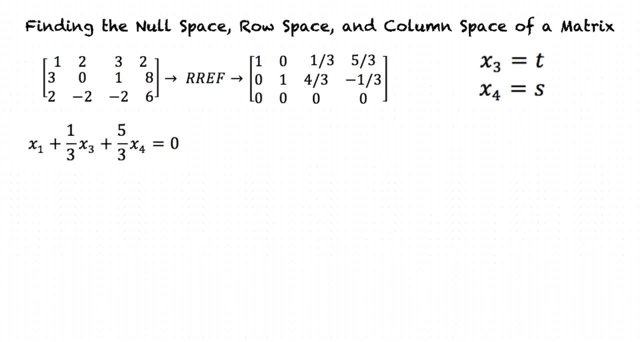 to 0.. We now substitute the variable t and s into the equation for x3 and x4. This will look like x1 plus 1 third t plus 5 thirds s is equal to 0.. Solve the equation so that it will look like x1 is equal to negative, 1 third t minus 5. 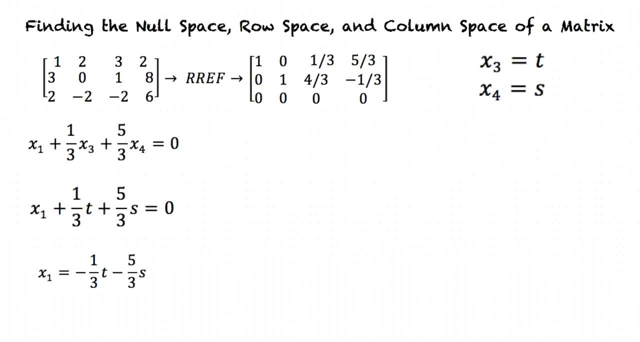 thirds s. Next we will solve for x2.. We start by solving the equation: x2 plus 4 thirds x3 minus 1 third, x4 is equal to 0.. Now substitute t and s in for x3 and x4. This will look like: x2 plus 4 thirds t minus 1 third s is equal to 0. 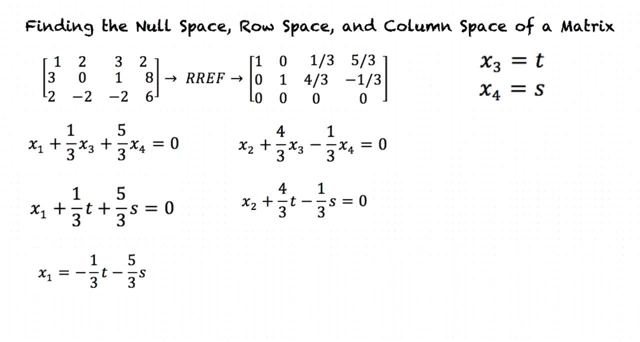 Now we solve the equation for x2.. Giving us x2 is equal to negative 4 third t plus 1 third s. Now that we have solved for x1 and x2, it is time to parameterize the solution so that 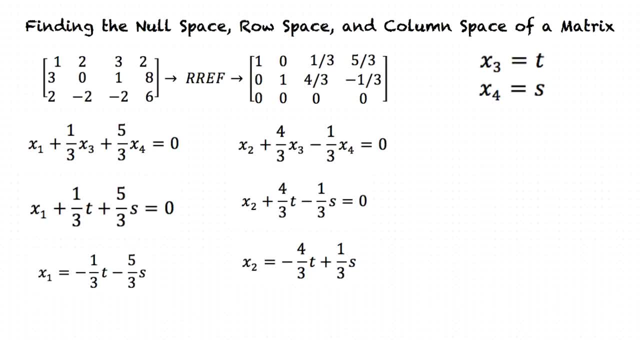 we can find the null space. So now, what do we do? Now we write the solution for each variable: x1 is equal to negative 1 third t minus 5 third s. X2 is equal to 3 thirds x3.. 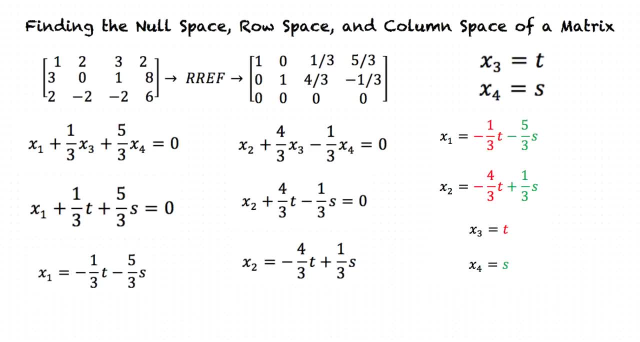 negative 4 thirds t plus 1 third s. x3 is equal to t and x4 is equal to s. We now take the span of all t variables and s variables. This will look like negative 1 third negative 4 thirds 1, 0,. 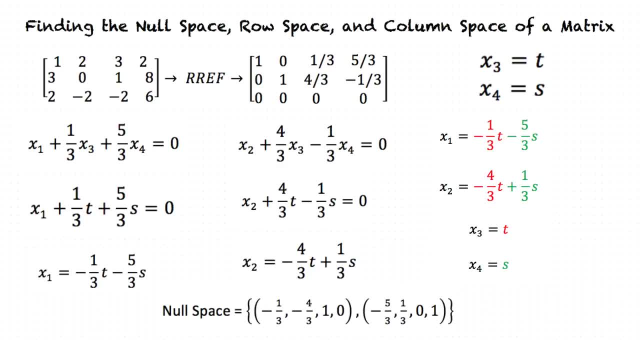 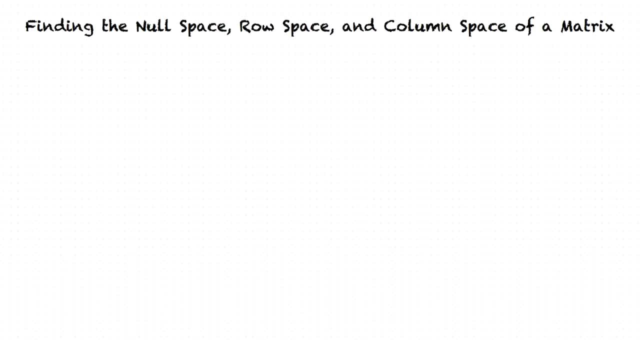 and negative 5 thirds: 1 third 0, and 1.. Our final solution for the column space, row space and the null space of matrix A is column space 1,, 3,, 2, and 2, 0, negative 2.. 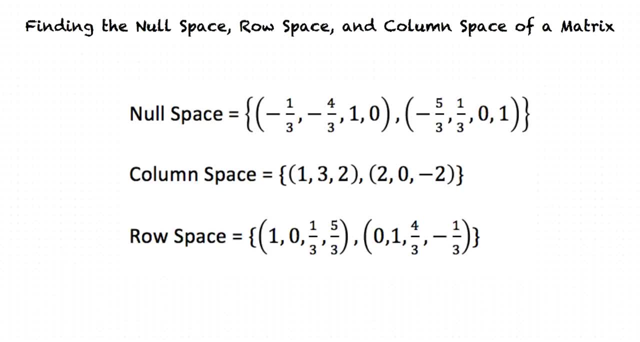 Row space: 1, 0,, 1 third, 5 thirds and 0, 1, 4 thirds and negative 1 third. For the null space: negative 1 third, negative 4 thirds, 1, 0,. 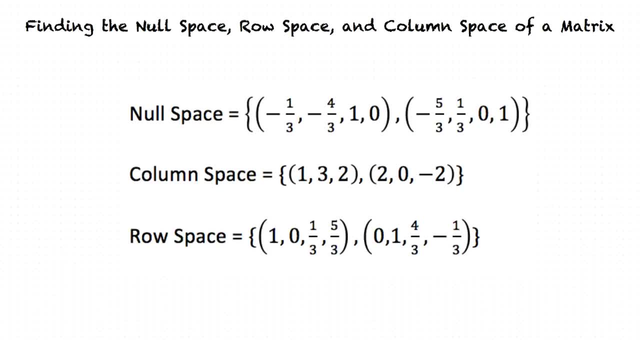 and negative, 5 thirds, 1 third 0, and 1.. This will be our final answer. Okay, I think I have it figured out. We first start by finding the reduced row echelon form of the matrix. From here we find the column space by finding the pivot points in the reduced row echelon form matrix.